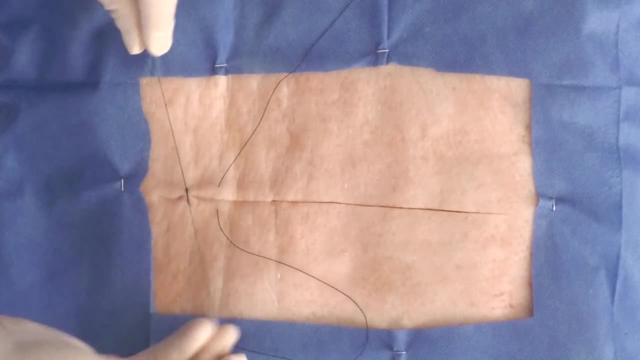 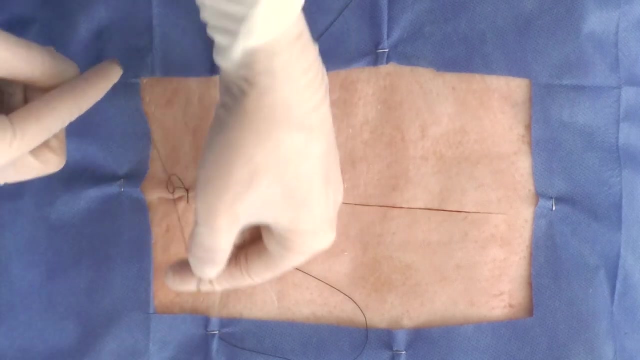 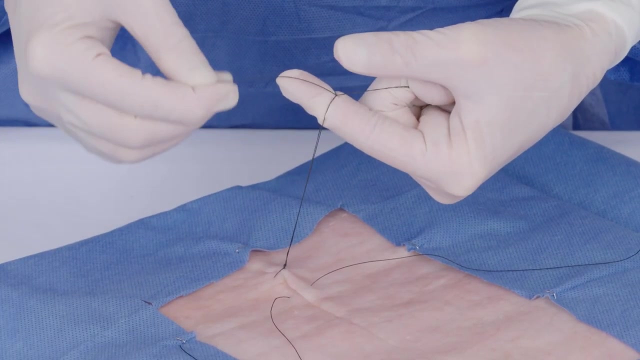 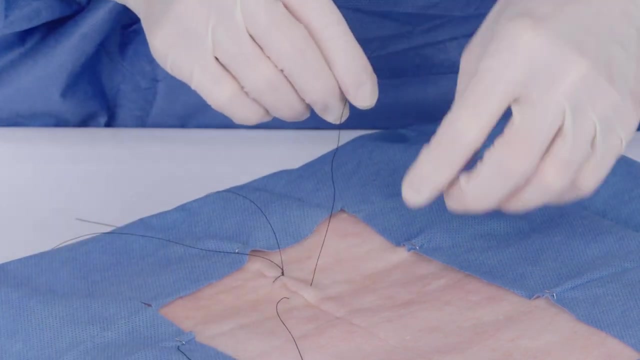 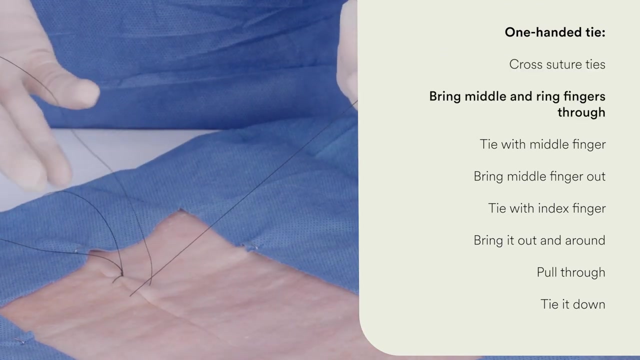 and tie it down. Index thumb, thumb through. tie it down, Thumb, index through. grab it with the index finger back through and tie it down For the one-handed tie. you're going to cross your suture ties. You're going to bring your. 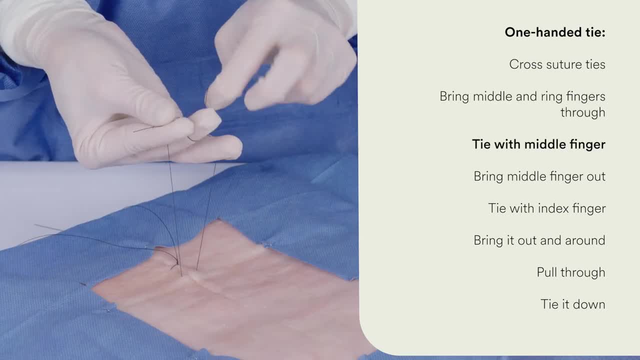 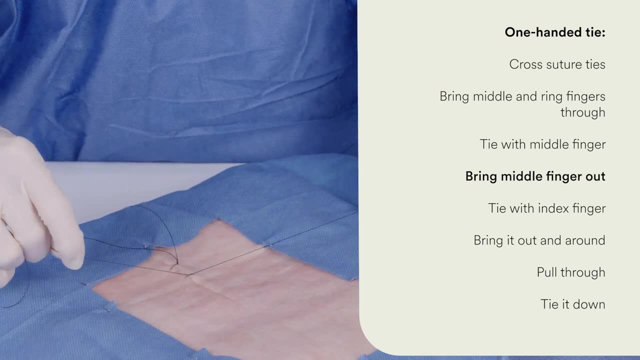 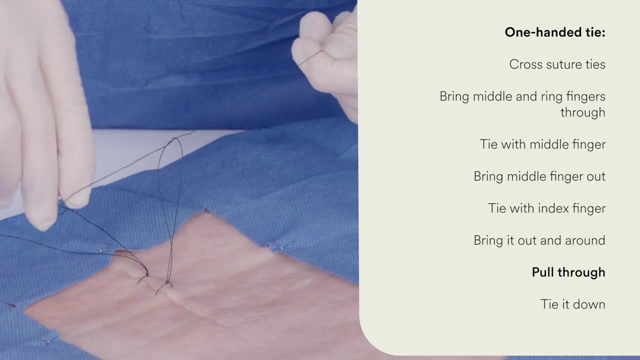 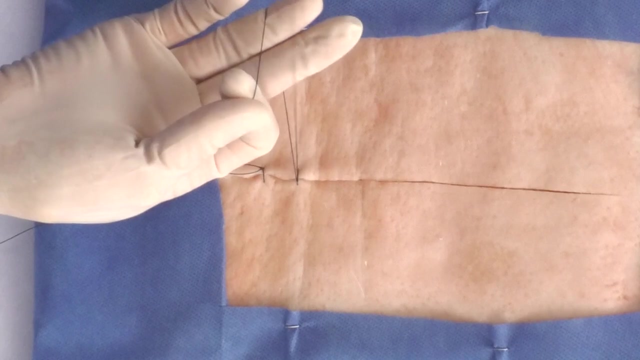 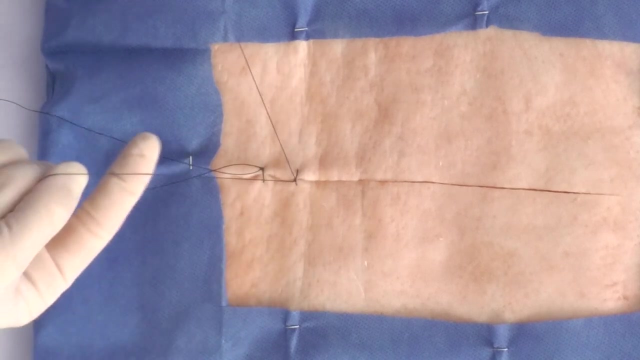 index finger and ring finger through. You're going to tie with your middle finger, Bring it out and down, And then now you're going to tie with your index finger, Bring it out around, through and tie. So again, this, this, this and down, this, this, this and down this, this, this and. 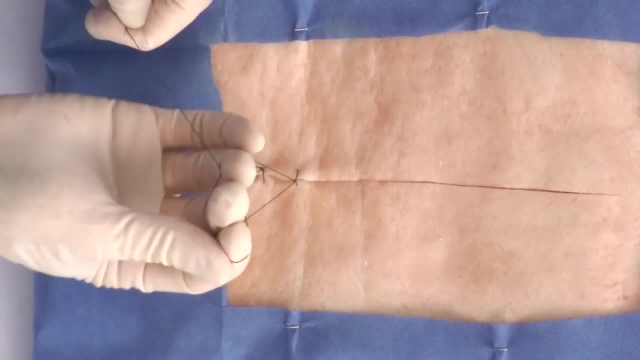 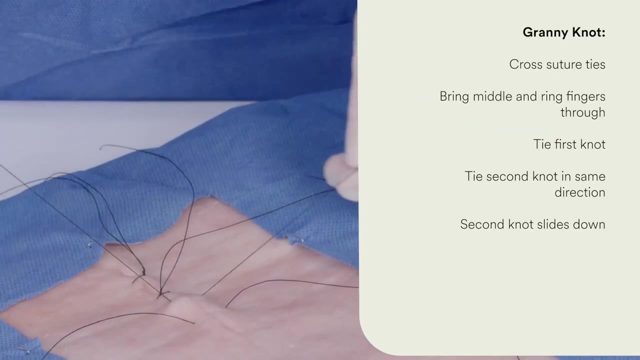 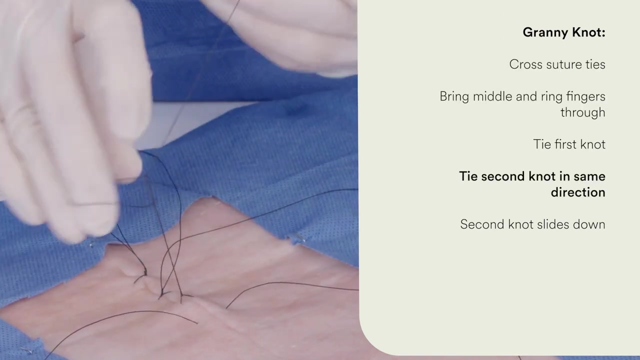 down. This little finger cross and down can do a granny knot, which means to do both knots in the same direction and they'll slide down. so do one knot in that direction and do another knot, and that knot will slide down. so 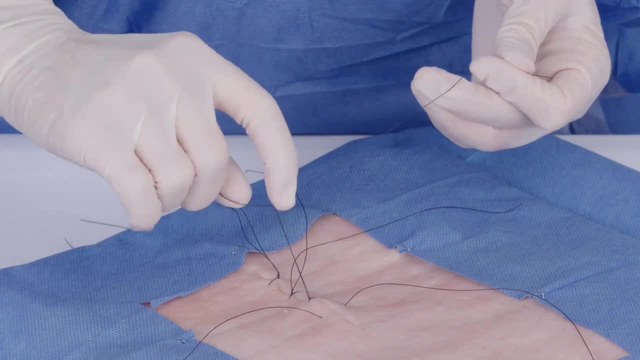 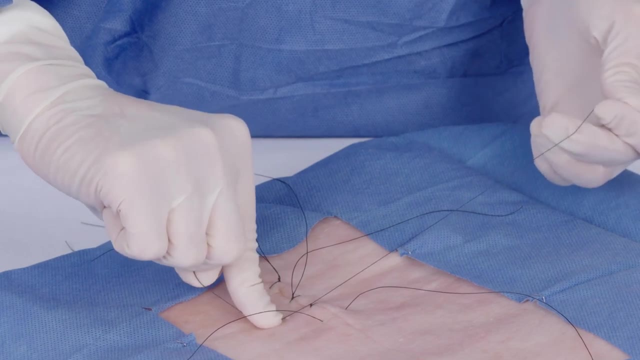 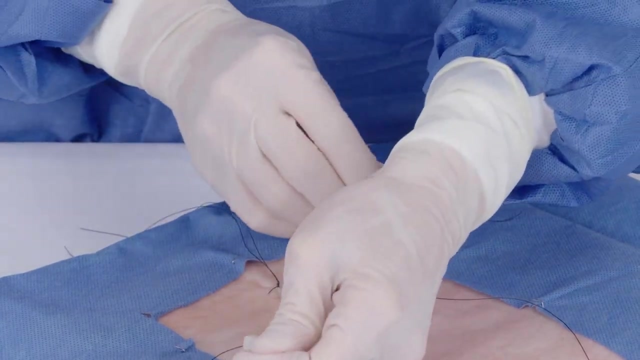 do it slower. so if i tie with my ring middle finger, put it down, i tie again with my middle finger two knots in the same direction. so they're not square and those sutures will tie down, will cinch down, and then you can start doing your square knots for that. 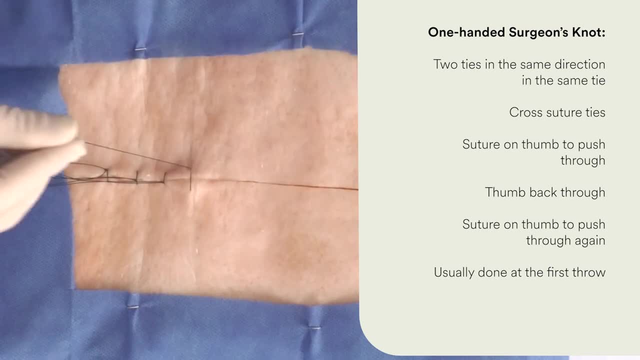 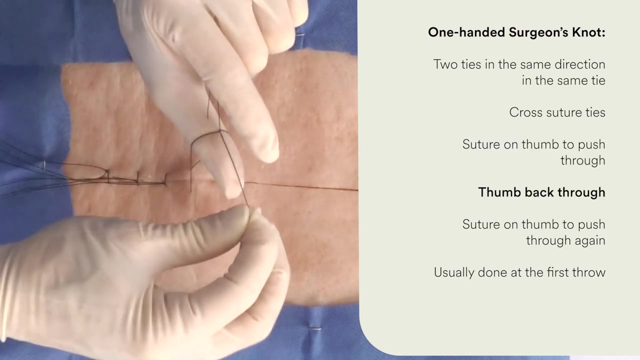 for a surgeon's knot. it means that you're going two ties in the same direction, all and in the same tie. so for one-handed, i've now put this on my thumb to push through. i'm going to go back through and push, put it on my thumb again and that's going to give me two knots. it's called the. 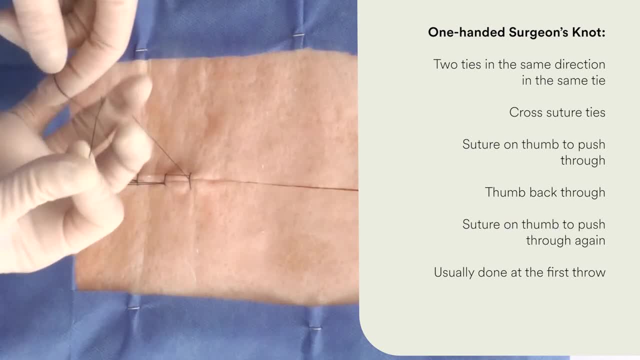 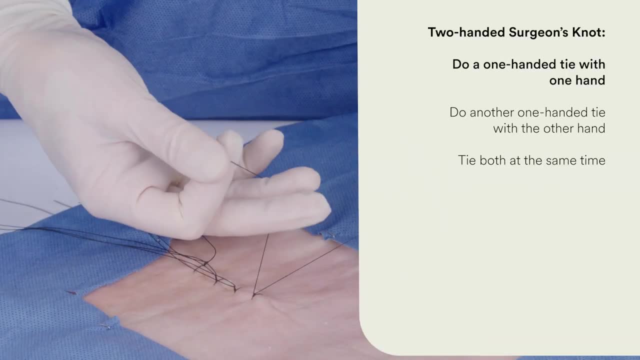 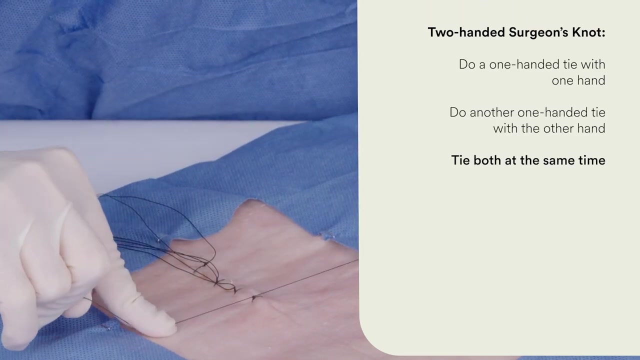 surgeon's knot, and usually that's done at the first throw and then we can do other things. you're going to be doing a one-handed tie with this hand and one-handed tie with that hand and do it all at the same time, and you get a surgeon's knot done with one throw rather than with the two.